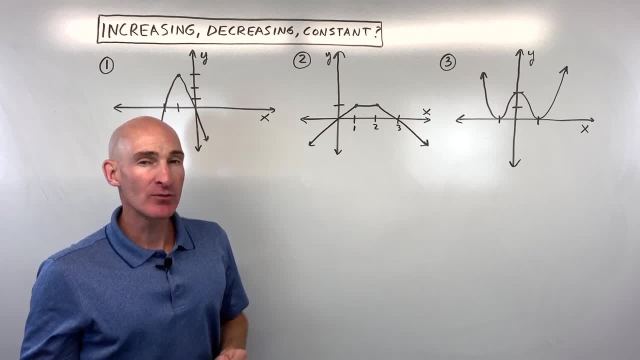 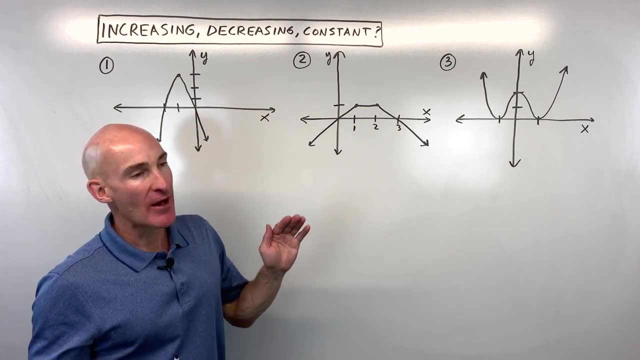 Now, if you don't remember anything at all from this video, the most important thing to remember is you don't want to include the endpoints of the interval, because what's happening is when the graph is changing from increasing to decreasing, or decreasing to increasing. 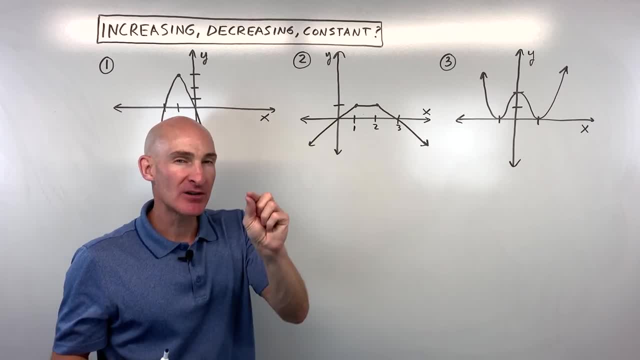 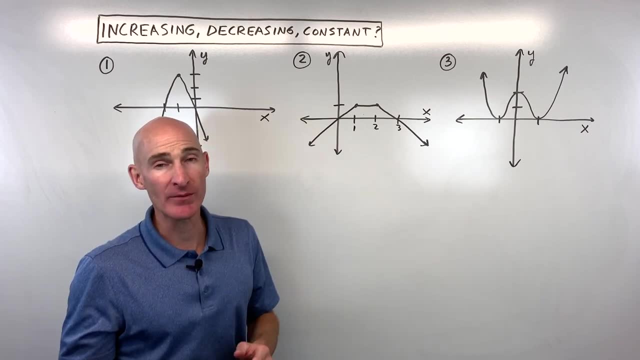 or decreasing to constant, whenever it's changing that particular point. where it's changing, you don't want to include it because it's kind of like it's switching, you know, from increasing to decreasing or one of the other types. So I'll show you what I mean. Let's go through some examples. 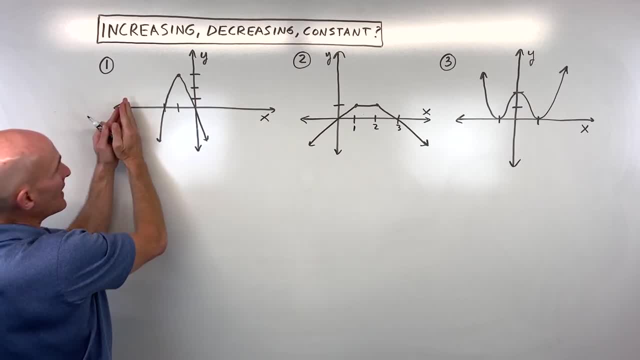 together. So for number one, what I would do is I would scan from left to right, just like I'm reading a book, And I'd say, oh, I can see the graph is going up to the right, So that tells me. 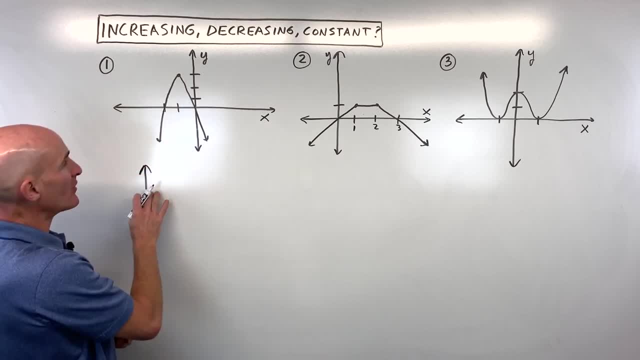 it's increasing, And I'll just draw an up arrow here to abbreviate increasing. And that's: for what values are the y values increasing? So for what x values are the y values going up, up, up? Well, that's going to be from negative infinity to negative one, And again, remember. 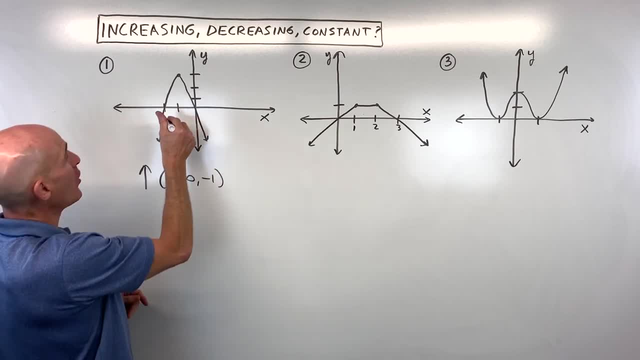 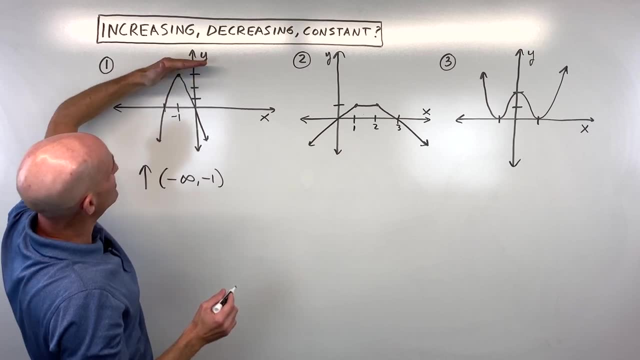 open interval. You don't want to include the endpoints because here, at negative one, you can see the graph is like: is it constant? Is it increasing? Is it decreasing? It's switching right. basically, at this point Now, where is the graph decreasing? 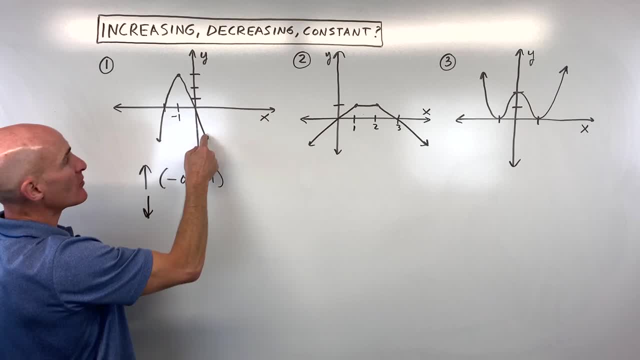 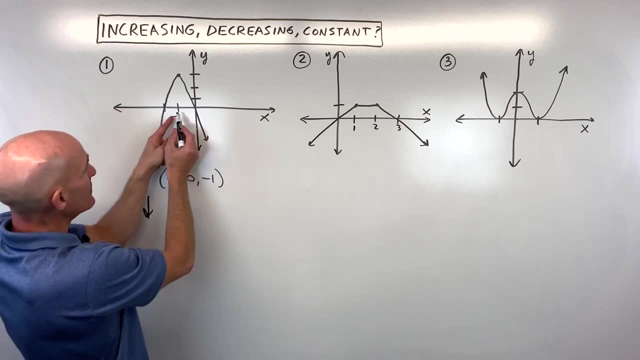 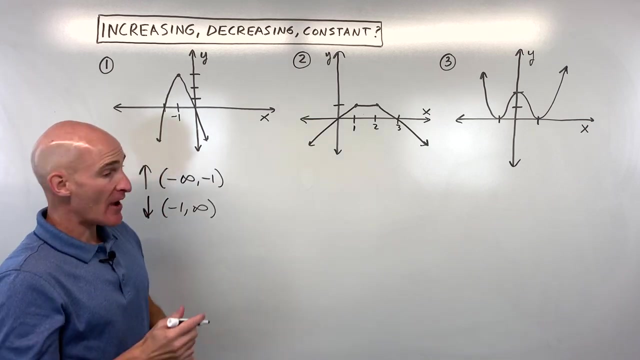 Well, again reading from left to right, the graph is going down, down, down. So we're basically saying: for what x values are the y values decreasing, And that's going to be from negative one to positive infinity, And again open intervals. And then where is the graph? 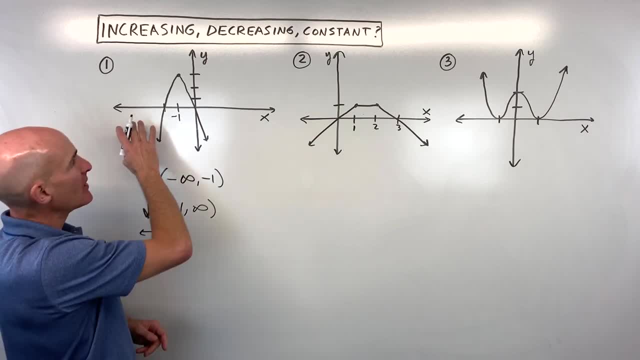 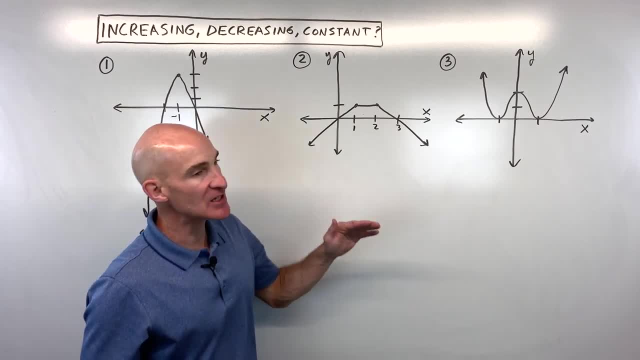 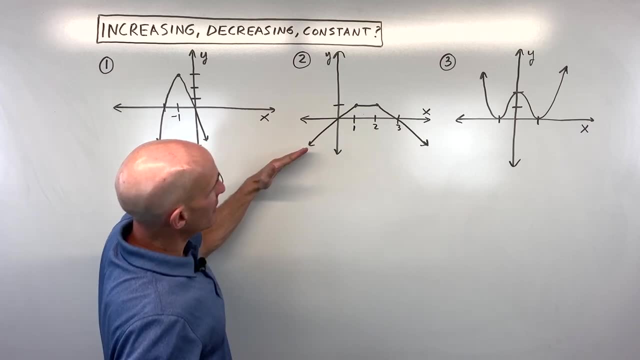 number two. So what do you think on this one? Where is the graph increasing, decreasing or constant? Well, again, reading kind of like a book, from left to right: okay, you can see that. okay, the graph's going up to the right. So, as x values, for what x values, are the y values increasing? Well, that's. 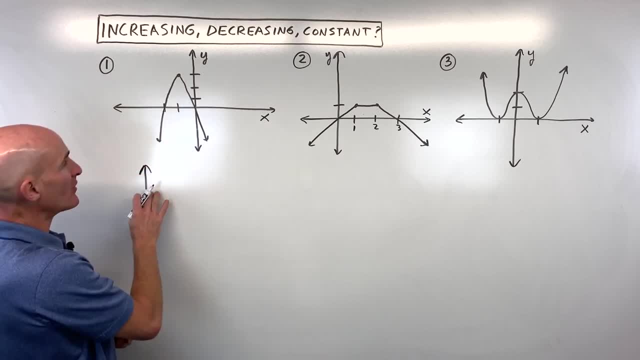 it's increasing, And I'll just draw an up arrow here to abbreviate increasing. And that's: for what values are the y values increasing? So for what x values are the y values going up, up, up? Well, that's going to be from negative infinity to negative one, And again, remember. 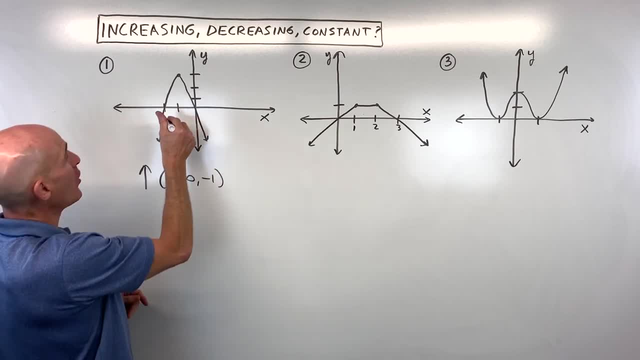 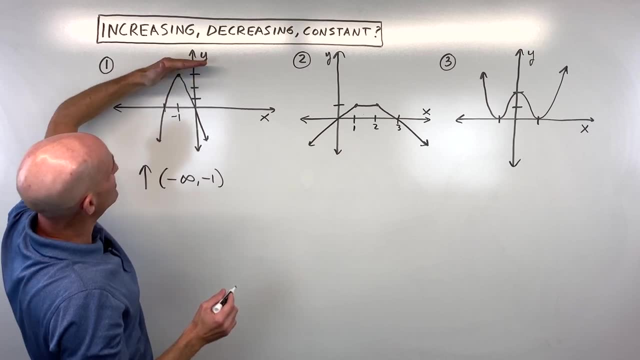 open interval. You don't want to include the endpoints because here, at negative one, you can see the graph is like: is it constant? Is it increasing? Is it decreasing? It's switching right. basically, at this point Now, where is the graph decreasing? 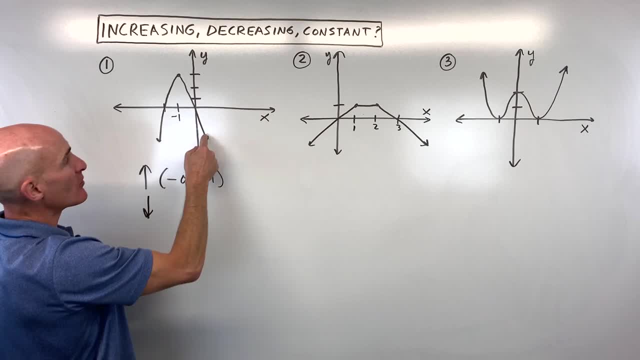 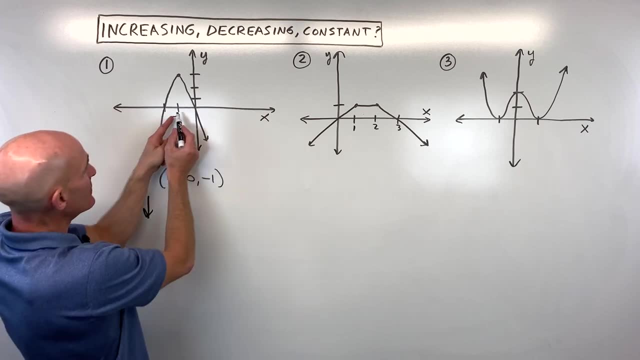 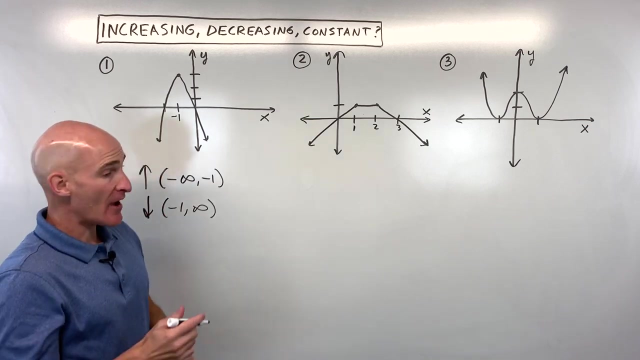 Well, again reading from left to right, the graph is going down, down, down. So we're basically saying: for what x values are the y values decreasing, And that's going to be from negative one to positive infinity, And again open intervals, And then where is the graph? constant. 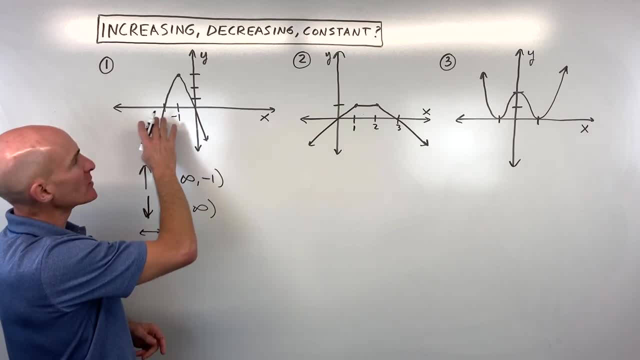 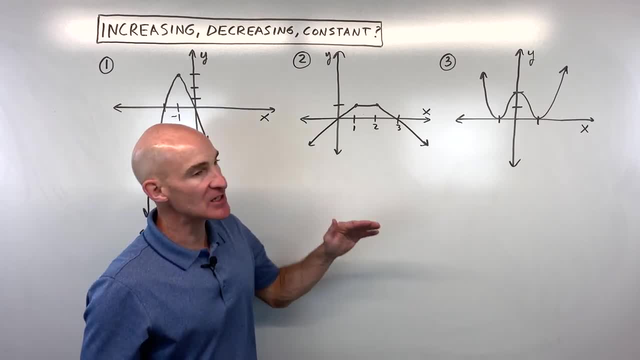 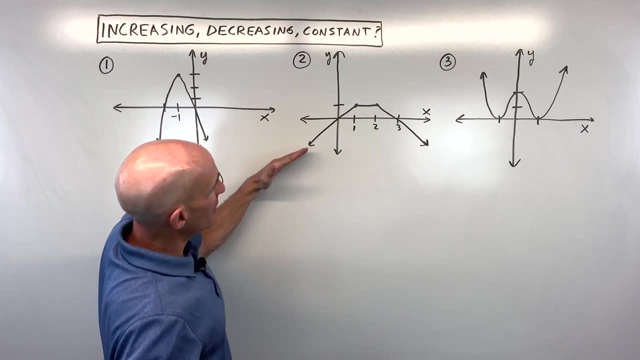 Number two. So what do you think on this one? Where is the graph increasing, decreasing or constant? Well, again, reading kind of like a book, from left to right. okay, you can see that. okay, the graph's going up to the right. So, as x values, for what x values are the y values? 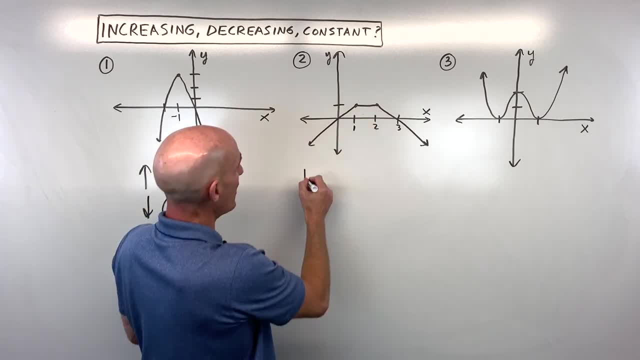 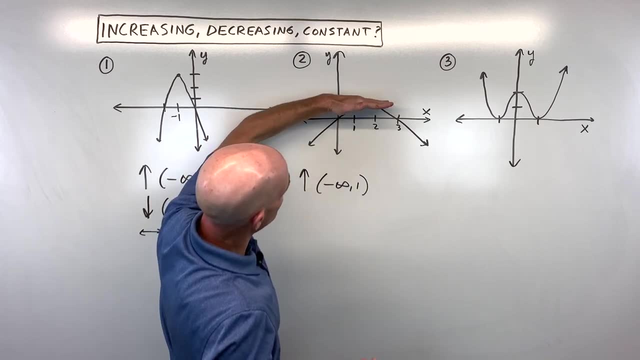 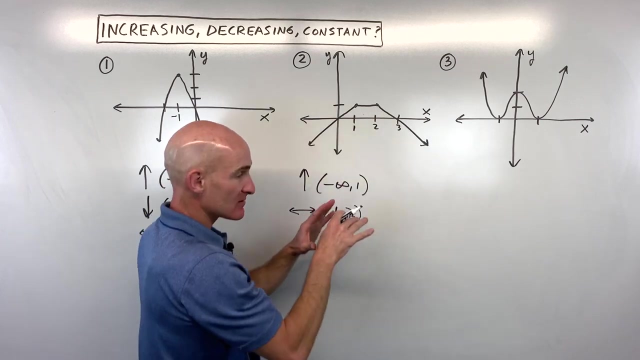 increasing. Well, that's from negative infinity to positive one, So negative infinity to positive one, not including one, because once you get to one you can see now we have a horizontal line, So it's going to be constant from one to two. Again, not including the end points, So open. 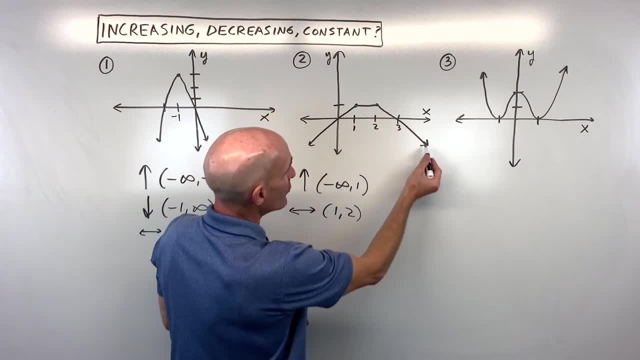 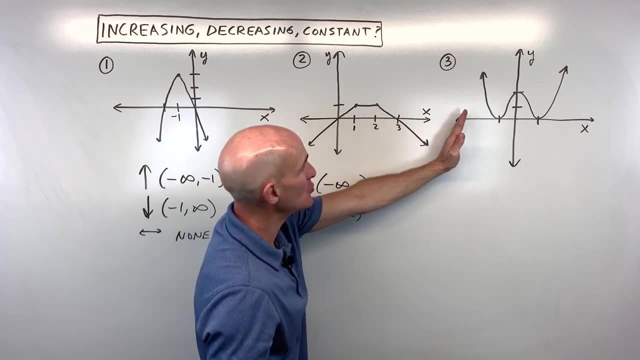 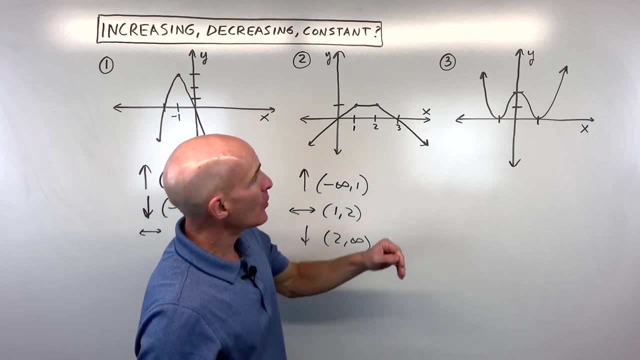 interval And then, once you get to two, it's going down to the right. That's like kind of like a negative slope, It's decreasing. So for what x values are the y values decreasing? That's from two onward, or we could say two to infinity. Okay, what do you think for number three? Where is the 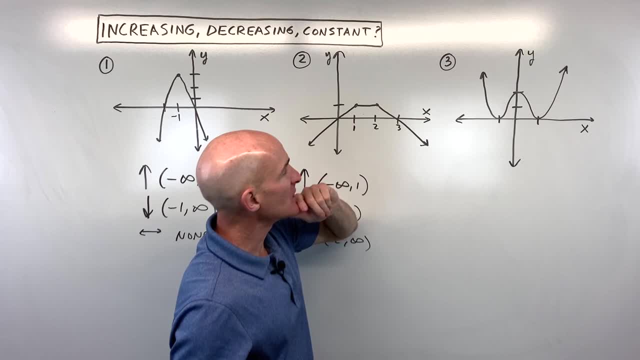 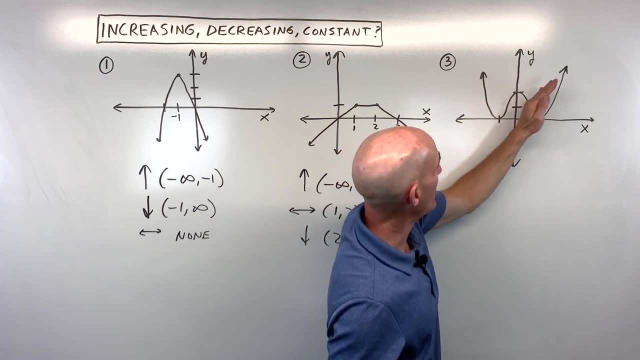 graph: increasing, decreasing, constant. Now this one's a little bit more challenging. So increasing I always think of like a slope, like a positive slope, So I know, like up to the right, up to the right. So basically, from here and here, these two little regions, it's increasing. 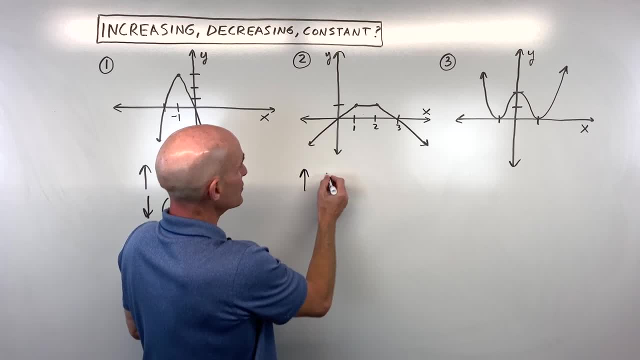 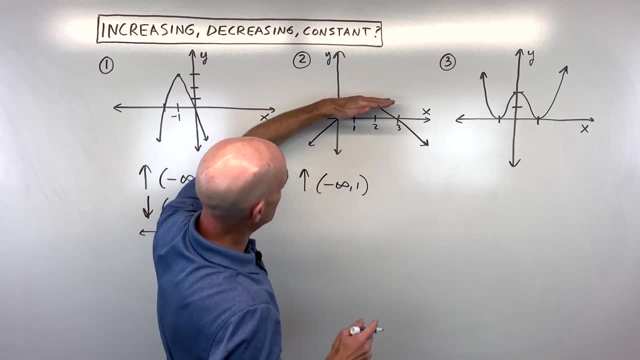 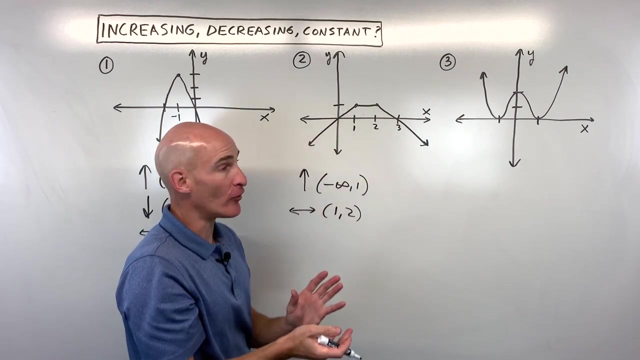 from negative infinity to positive one, So negative infinity to positive one, not including one, because once you get to one you can see now we have a horizontal line, So it's going to be constant from one to two, again not including the end points. so open interval and then, once you get, 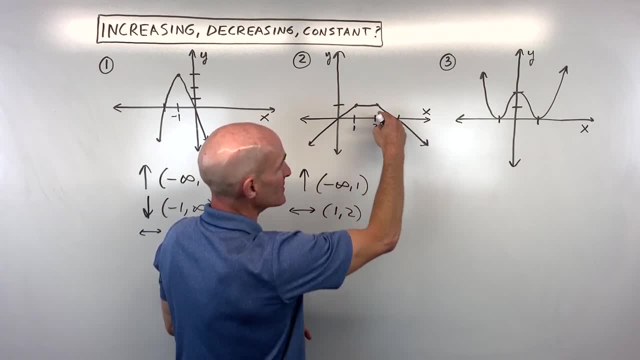 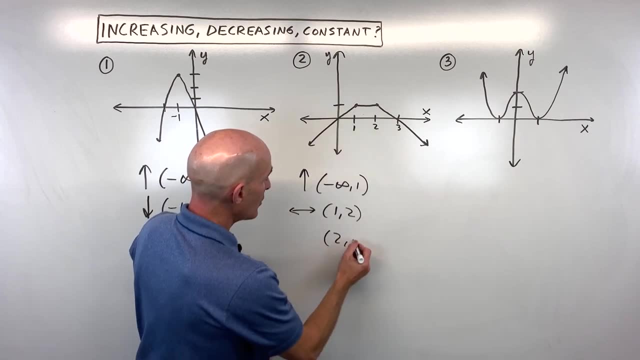 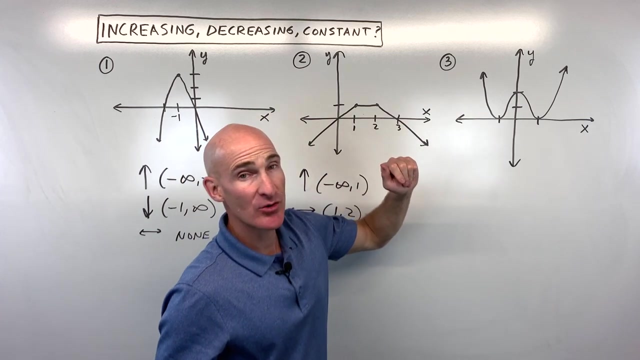 to two. it's going down to the right. That's like kind of like a negative slope, it's decreasing. So for what x values are the y values decreasing? That's from two onward, or we could say two to infinity. Okay, what do you think for number three? Where is the graph? increasing, decreasing? 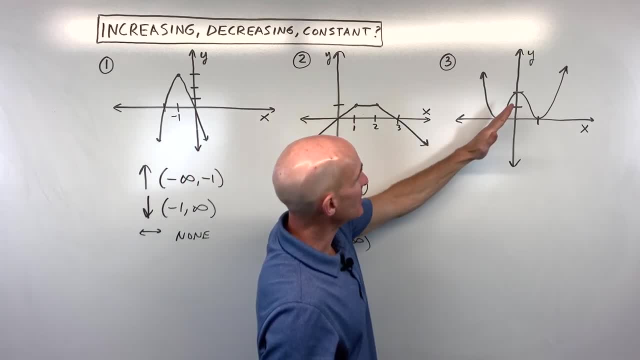 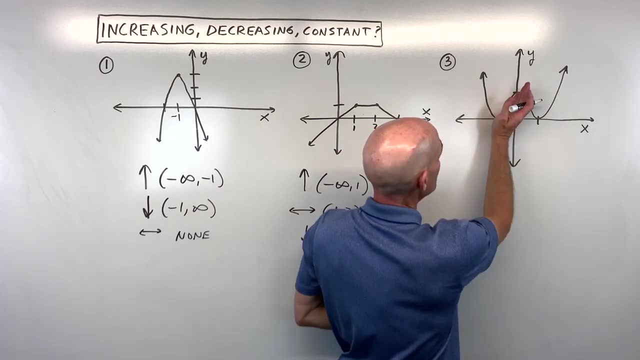 constant. Now this one's a little bit more challenging. So increasing I always think of like a slope, So increasing, decreasing constant. So increasing constant, So increasing constant, So from one to one is increasing. So what we're going to do for increasing on this one is we're. 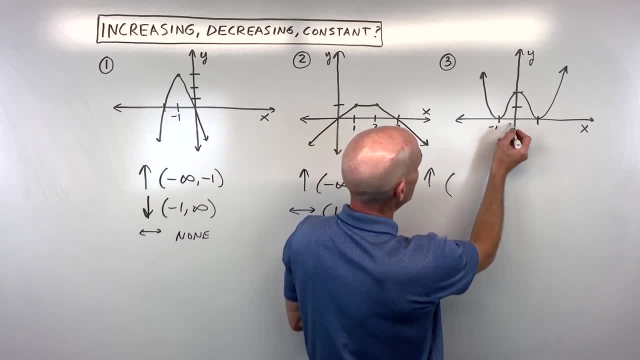 going to say from one- sorry negative one to zero. okay, it's increasing. But also from one onward, it's increasing. So we're going to put the? u for union and we have two intervals united together. Make sure you work from positive. we want it to be a beautiful and ridiculous device. okay, And I hope. 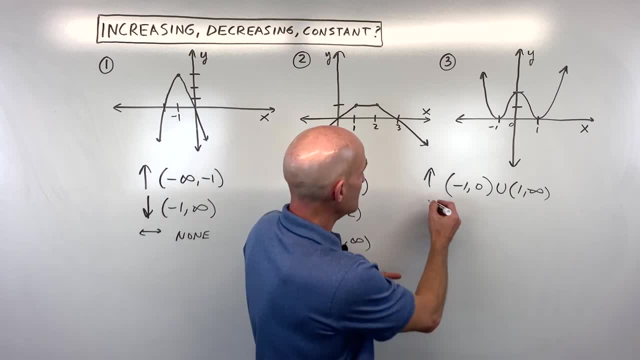 you are doing alright, from left to right, like low to high. Now where is the graph decreasing, meaning it's going down to the right, kind of has like a negative slope. We can see here it's going down to the right. 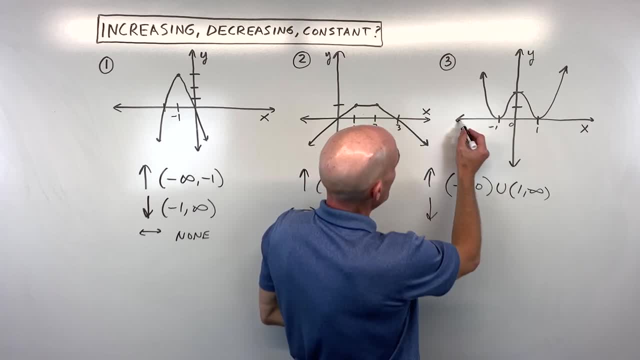 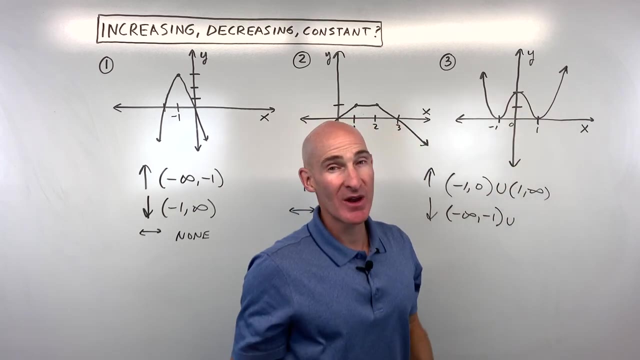 here it's going down to the right. So again two intervals. and so for what x values are the y values decreasing? That's gonna be from negative infinity to negative one again, not including the end points, union from zero. Now see, here's where students make a mistake. 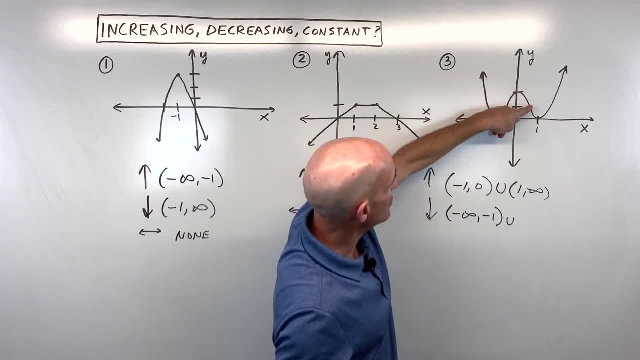 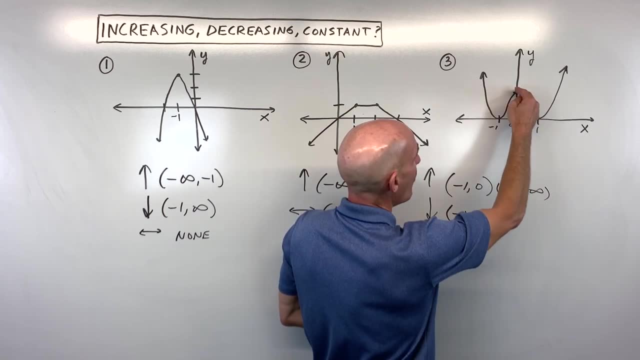 They sometimes look at the y values and say, oh, it's decreasing from two down to zero. Those are the y values. so I always say to myself: for what x values are the y values decreasing? So the y values are going down between zero and one. 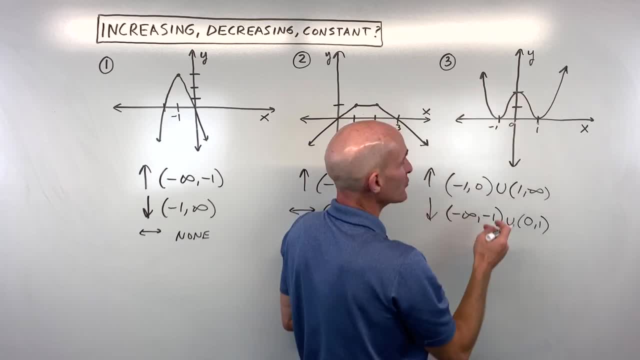 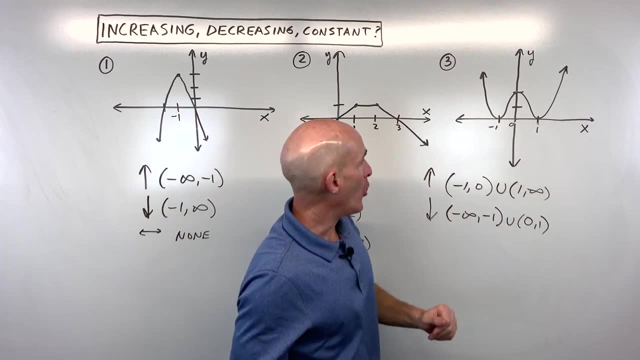 Again using an open interval. it doesn't include zero, doesn't include one, because at those points it's then changing direction. And is there any place on this graph where it's horizontal or constant? No, it would look something more like this: 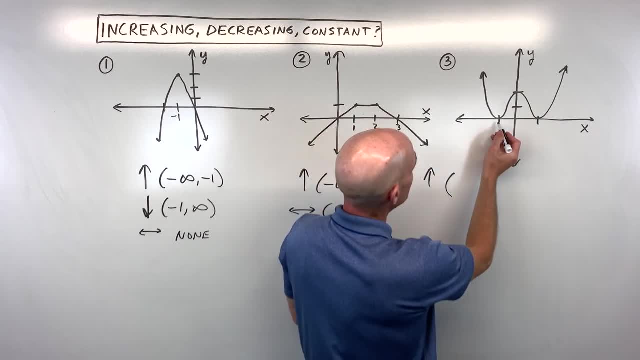 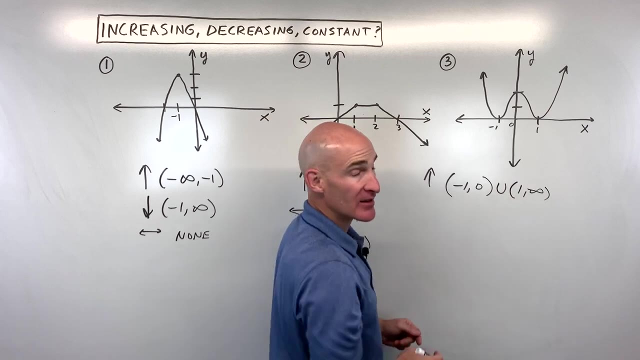 So what we're going to do for increasing on this one is we're going to say from one sorry negative one to zero, Okay, it's increasing. but also from one onward it's increasing. So we're going to put the u for union And we have two intervals united. 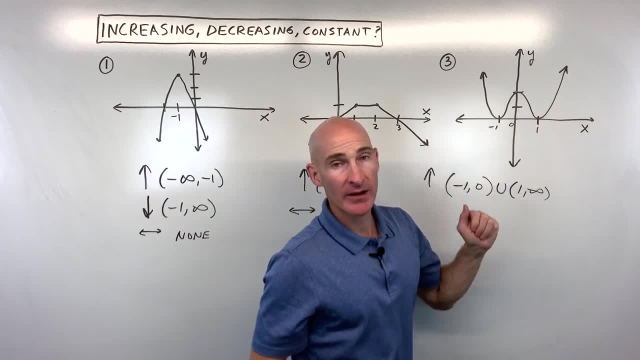 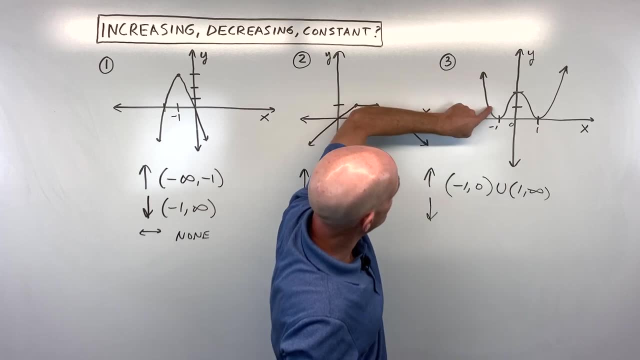 okay, together, Make sure you work from left to right, like low to high. Now where is a graph decreasing, Meaning it's going down to the right, kind of has like a negative slope. We can see, here it's going down to the right, here it's going down to the right. So again two intervals, And so for what? 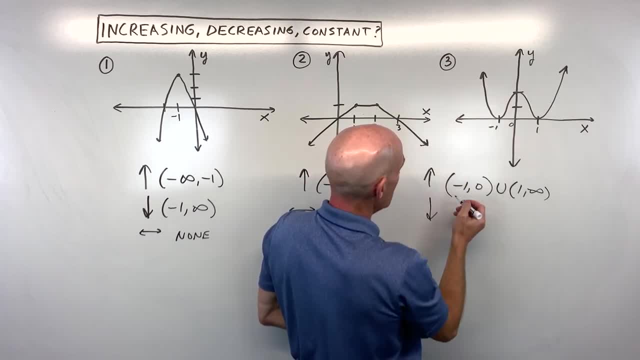 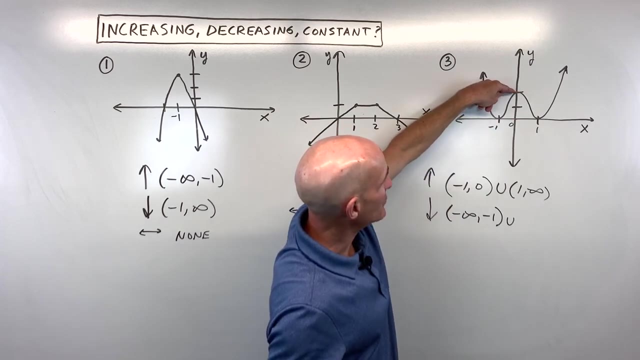 x values are the y values decreasing. That's going to be from negative infinity to negative one again, not including the endpoints union from zero. see this Now. see here's where students make a mistake. They sometimes look at the y values and say, oh, it's decreasing from 2 down to 0.. 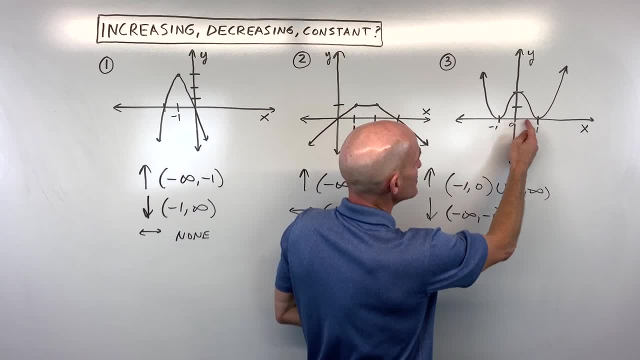 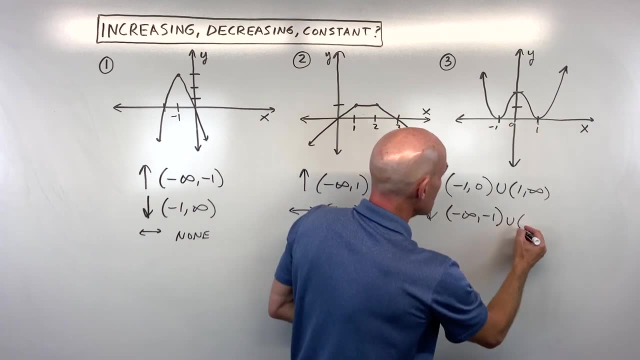 Those are the y values. So I always say to myself: for what x values are the y values decreasing? So the y values are going down between 0 and 1.. Again, using an open interval. it doesn't include 0,. it doesn't include 1,. 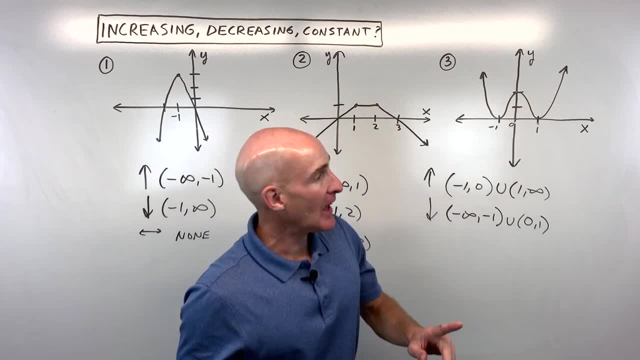 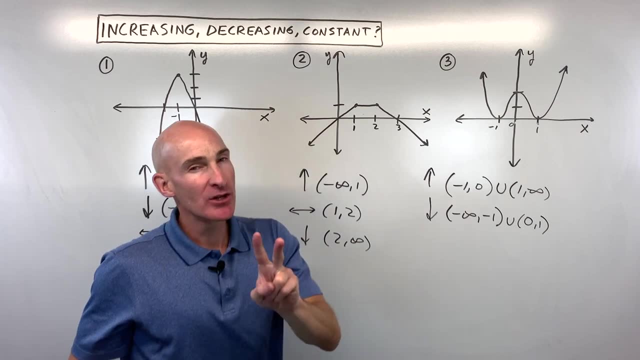 because at those points it's then changing direction. And is there any place on this graph where it's horizontal or constant? No, It would look something more like this, like a horizontal line. So let's do two more examples together. Maybe you can pause the video and try these on your own for some practice. 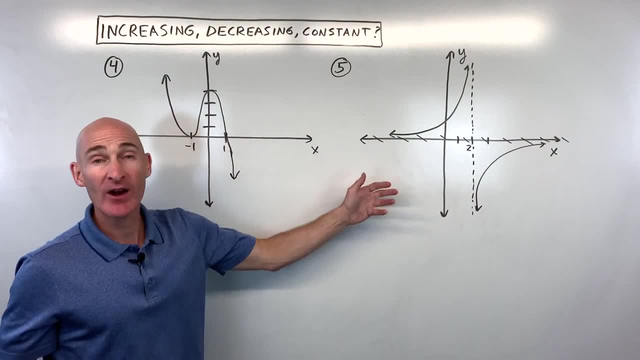 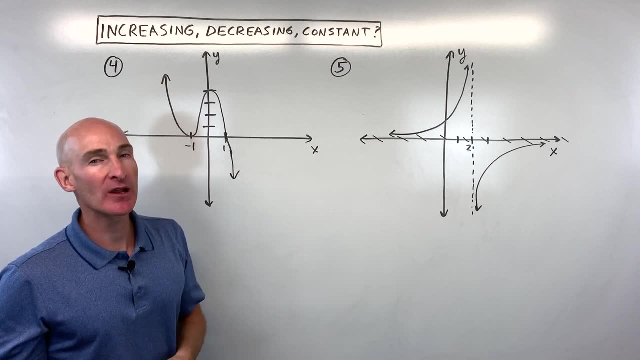 and let's look at those next. Okay, so what do you think for number 4 and 5?? Where is the graph increasing, decreasing or constant in interval notation? See, if you can do these, And while you're doing that, I just want to let you know. 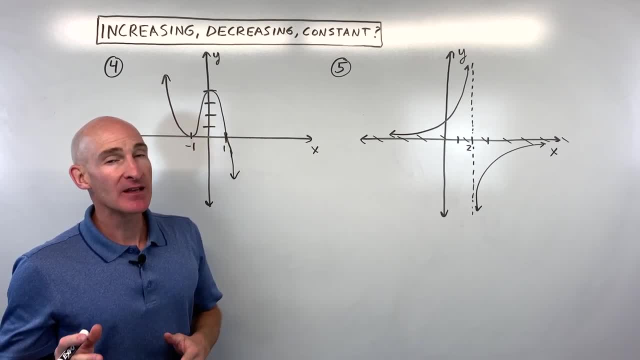 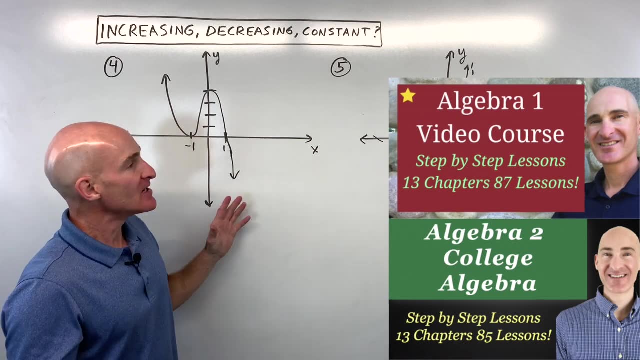 if you like the way that I explain things. I've got video courses for sale on Algebra 1 and Algebra 2, slash College Algebra. And what's neat about these courses is that sometimes in my videos I highlight some of the You know. 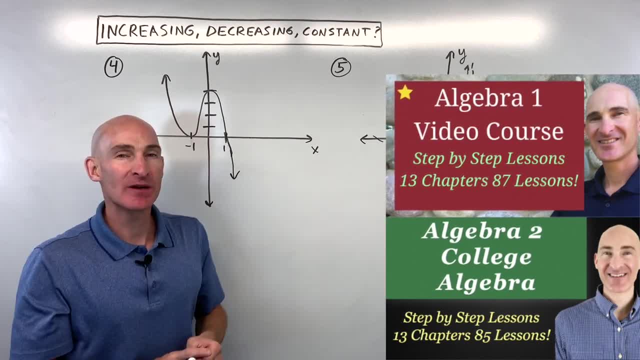 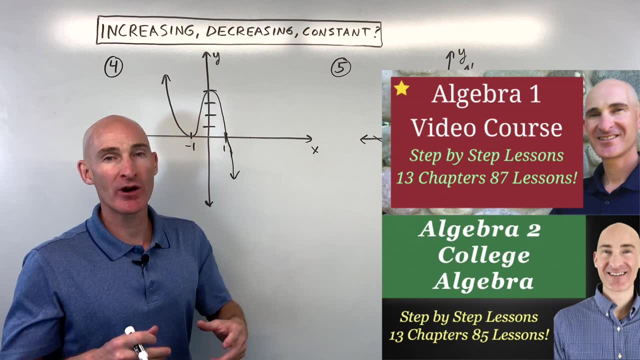 important concepts, but there's some connecting concepts sometimes that don't get covered in my YouTube videos or even in other YouTube videos, because people are highlighting, oh, how to complete the square or how to graph a parabola, But sometimes there's some little in-between. 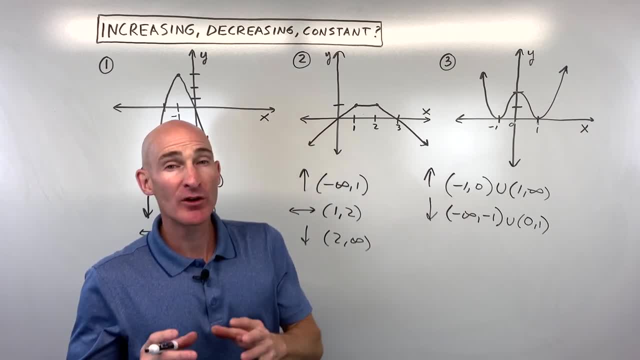 like a horizontal line. So let's do two more examples together. Maybe you can pause the video and try these on your own for some practice. and let's look at those next. Okay, so what do you think for number four and five? 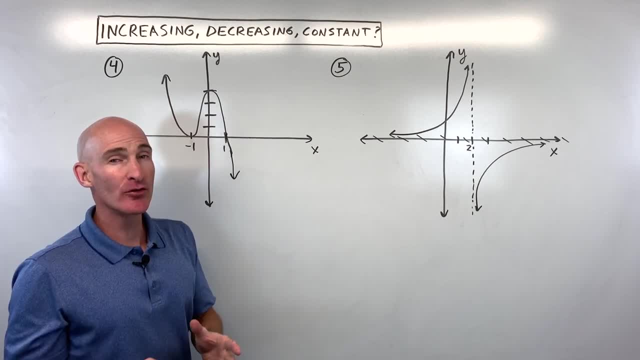 Where is the graph increasing, decreasing or constant in interval notation? See if you can do these. and while you're doing that, I just wanna let you know if you like the way that I explain things. I've got video courses for sale. 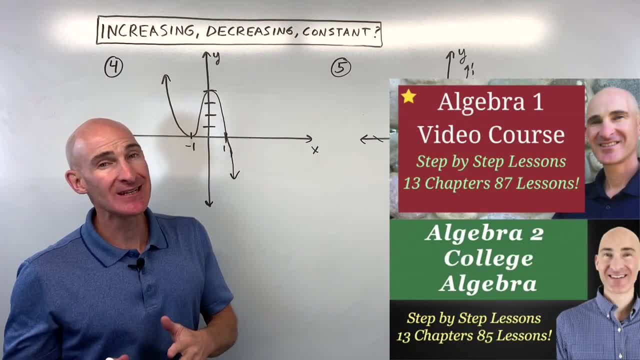 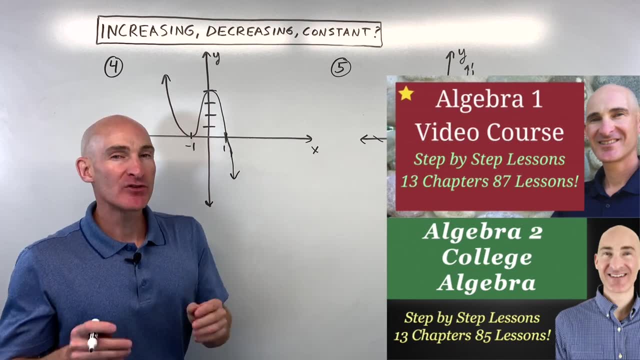 on Algebra 1 and Algebra 2- slash College Algebra, and what's neat about these courses is that sometimes in my videos I highlight some of the important, important concepts, but there's some connecting concepts sometimes that don't get covered in my YouTube videos. 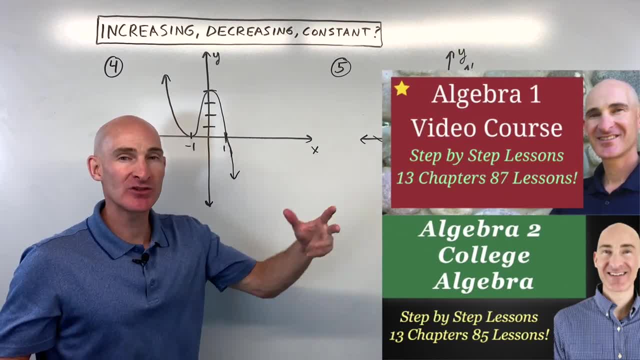 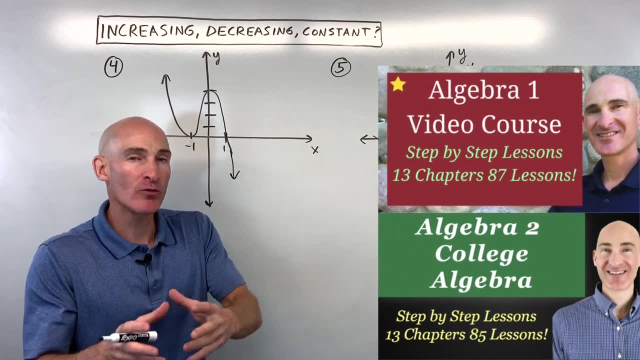 or even in other YouTube videos, because people are highlighting, oh, how to complete the square or how to graph a parabola. but sometimes there's some little in between, I would say, kind of like connectors that help you to build from one concept onto the next. 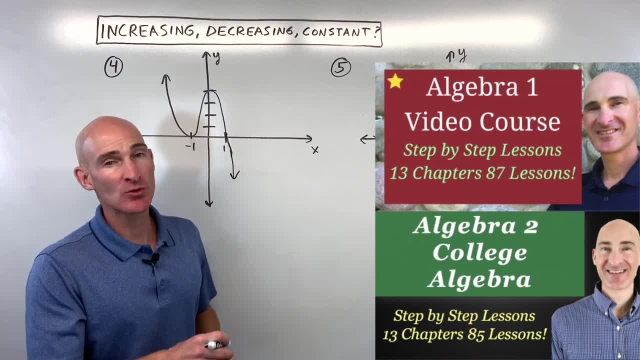 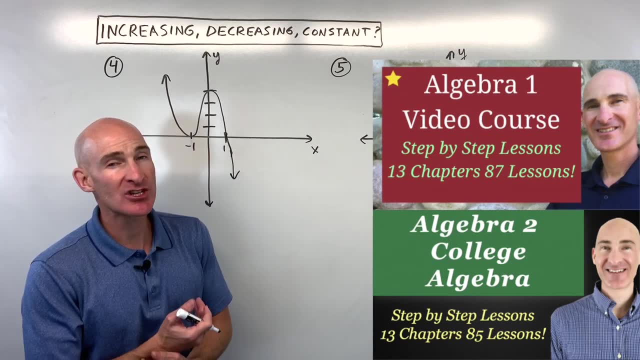 and those are the types of things that I talk about in the courses, as well as those key concepts as well, building one concept on top of it to the next. So, if you like the way I explain things, check out those courses for sale. 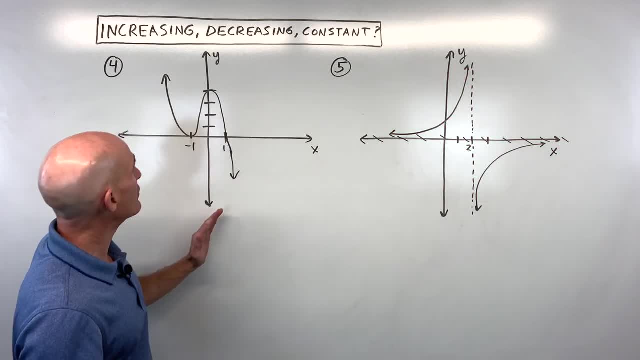 video links in the description. and what do you think for number four and number five now? So where is the graph increasing Now? another analogy that might help you is: imagine you're driving a car, okay, so here's your little car, okay. 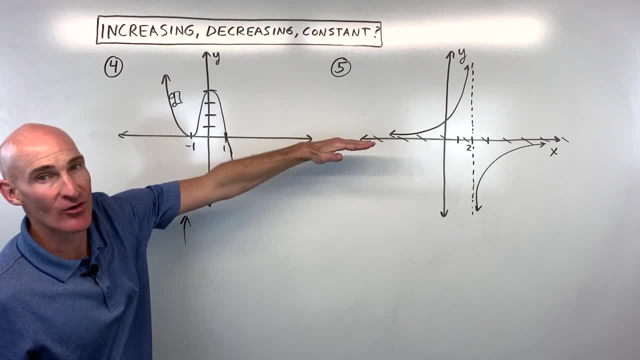 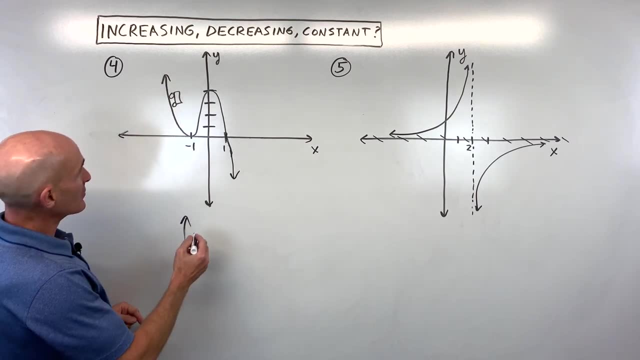 and you drive the car from left to right like this across the graph, So you can see that it makes sense that we're going downhill right, And so that means, okay, that's decreasing, that's decreasing here the car is going. 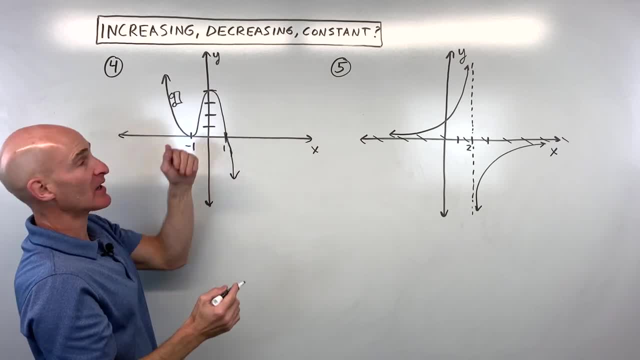 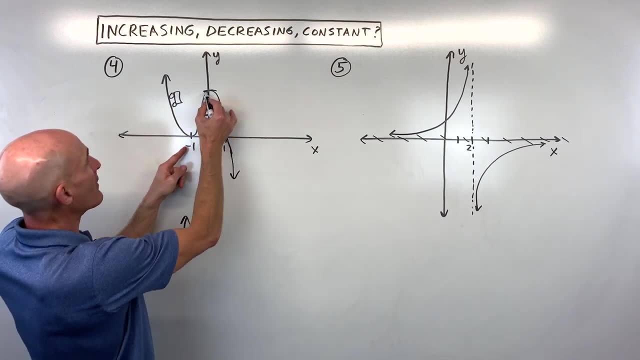 up to the right, like it's going uphill, okay, kind of like a roller coaster here. So it looks like it's increasing from negative one to zero. So for what x values are the y values going up? That's from negative one to zero. 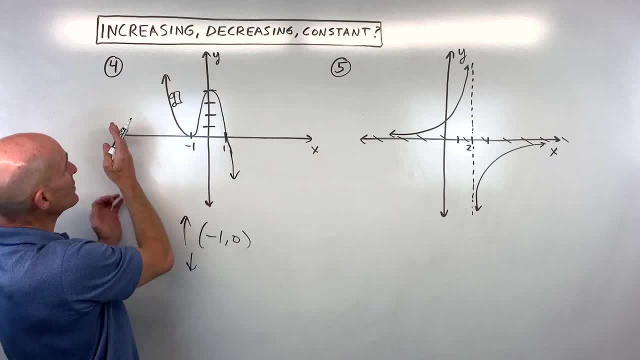 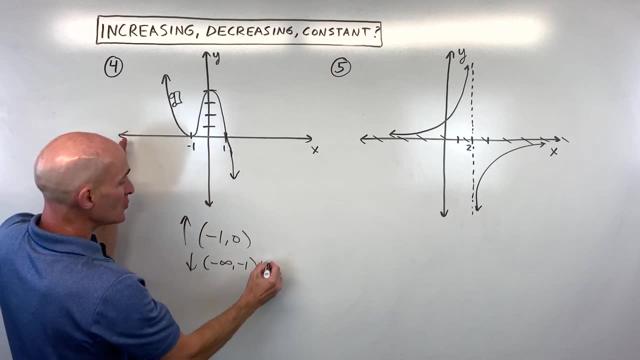 Again, remember open intervals. Where is the graph decreasing? Well, you can see from negative infinity to negative one. remember we're using the x values. and then union, also from zero onward, so we can say from zero to zero. 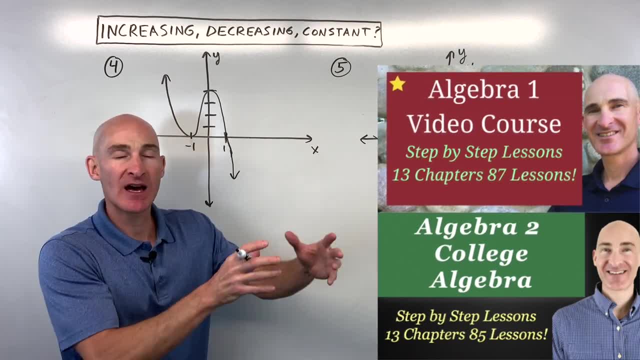 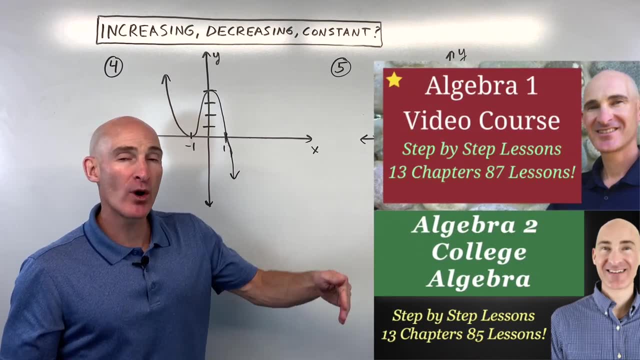 I would say, kind of like connectors that help you to build from one concept onto the next. And those are the types of things that I talk about in the courses, as well as those key concepts as well: building one concept on top of it to the next. 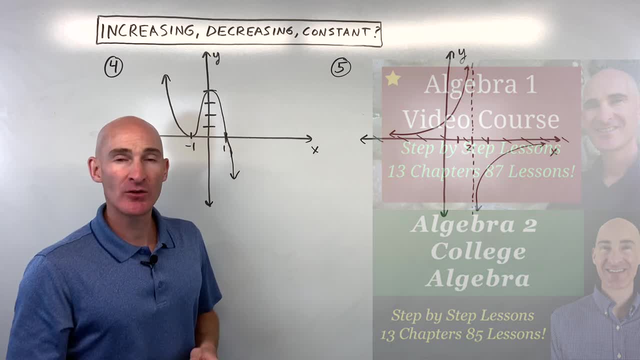 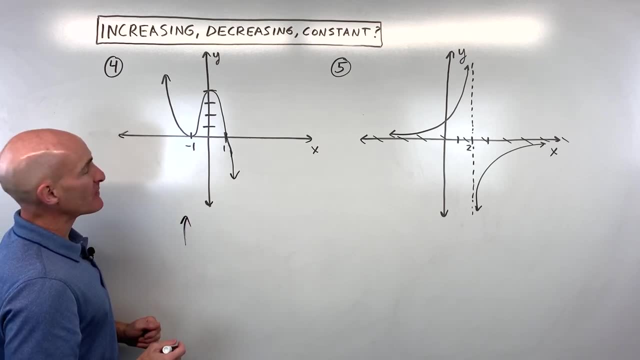 So, if you like the way I explain things, check out those courses For sale video links in the description. And what do you think for number four and number five now? So where is the graph increasing Now? another analogy that might help you is: 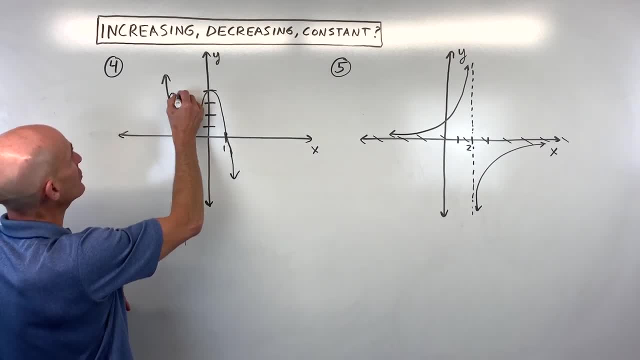 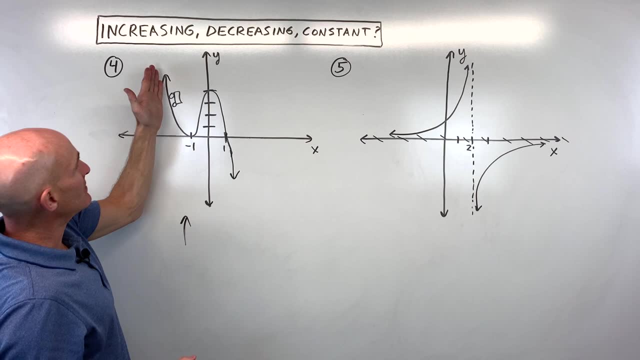 imagine you're driving a car, Okay. so here's your little car, Okay, And you drive the car from left to right like this across the graph. So you can see that it makes sense that we're going downhill, right, And so that means. 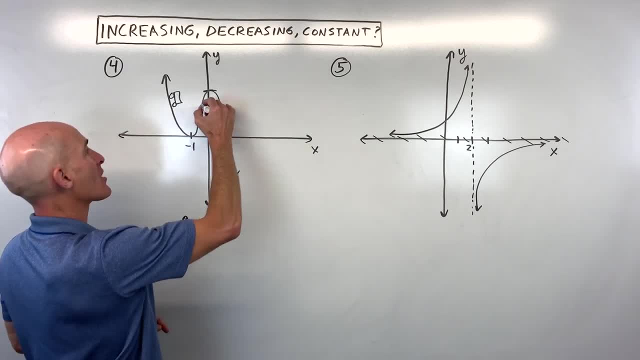 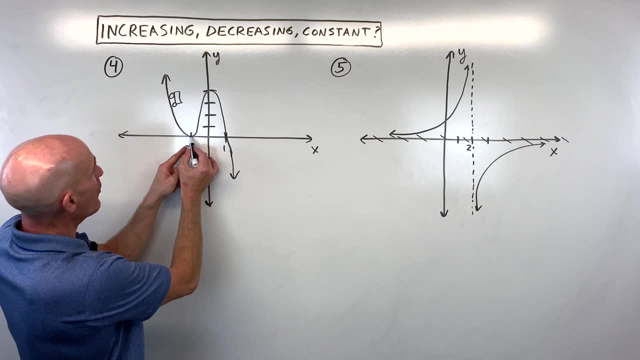 okay, that's decreasing. that's decreasing. Here the car is going up to the right like it's going uphill- Okay, kind of like a roller coaster here. So it looks like it's increasing from negative one to zero. 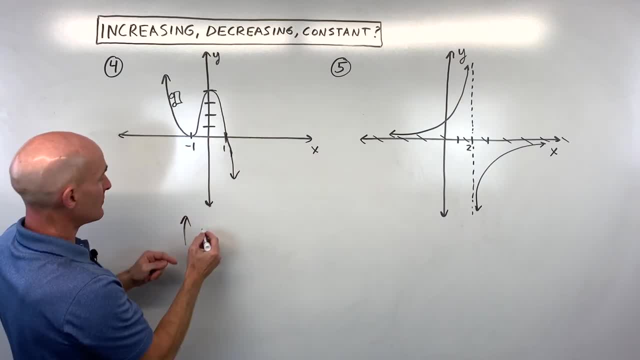 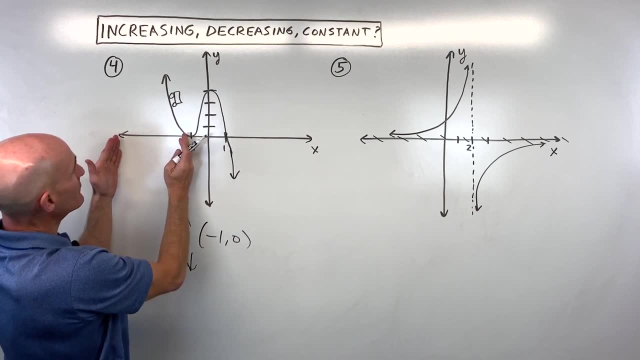 So for what x values are the y values going up? That's from negative one to zero. Again, remember open intervals. Where is the graph decreasing? Well, you can see from negative infinity to negative one. Remember we're using the x values. 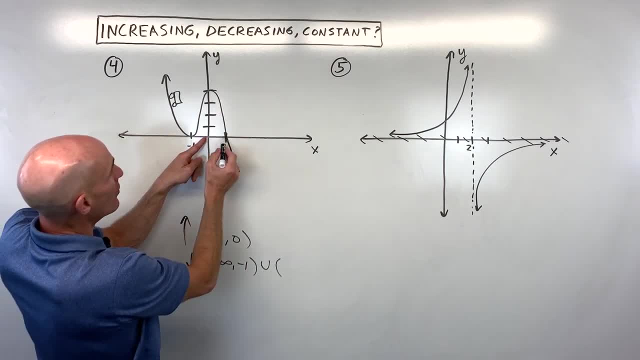 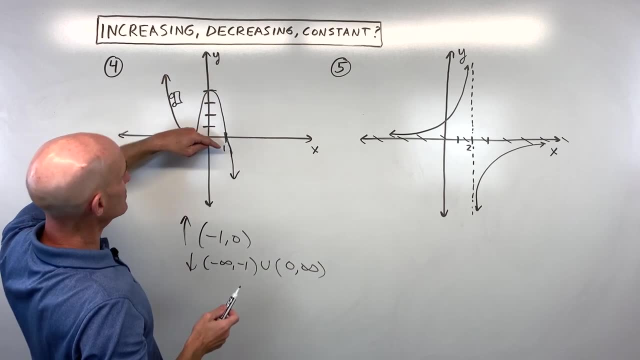 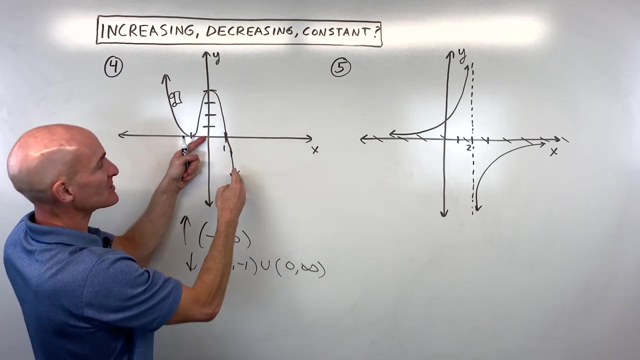 And then union, also from zero onward, So we can say from zero to positive infinity. Again, don't want to be confused and say, oh, from four to negative infinity or negative infinity to four. Those are the y values We're saying. for what x values are? the y's going down? 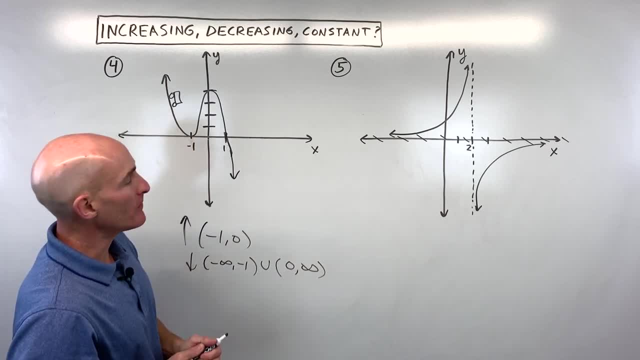 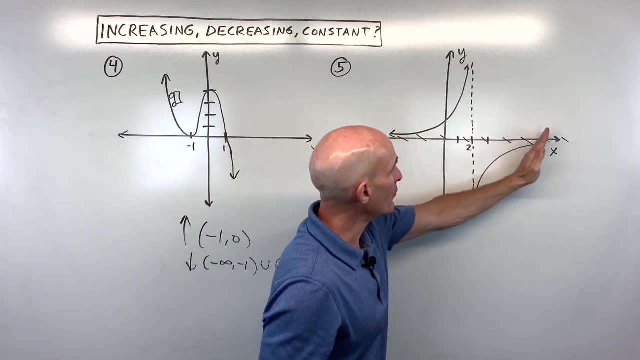 down, down, down. Okay For number five. what did you get for this one? Where is the graph increasing, decreasing or constant? Well, again, you want to think about going from left to right and think about this graph is going. 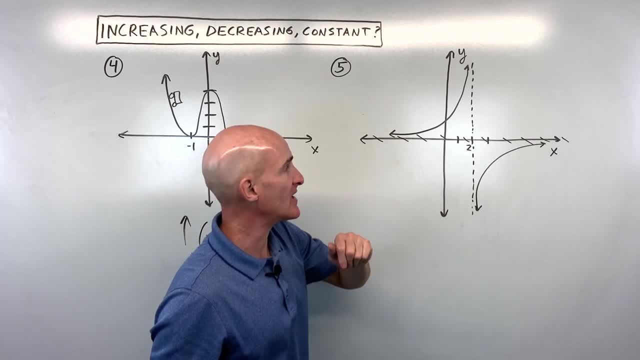 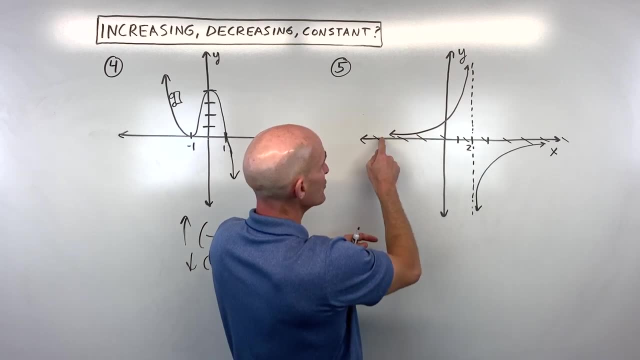 if it's up to the right, it's increasing down to the right, decreasing horizontal constant. What's interesting about this graph is we've got- it's got- some asymptotes. See these dashed or dotted lines. So the graph's going to get closer to those asymptotes. 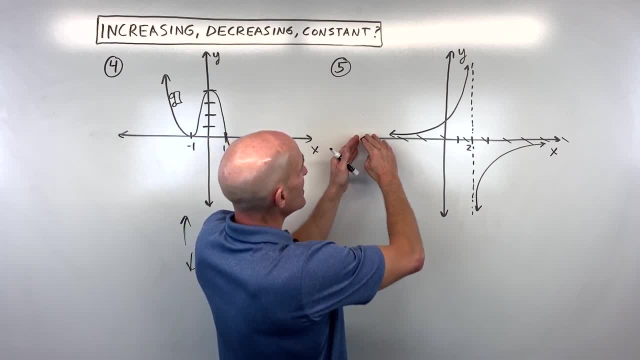 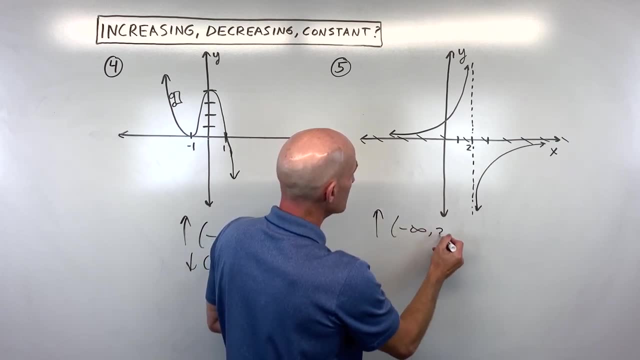 but it's not going to touch, Not going to cross. So here it looks like it's increasing, basically from negative infinity to two- Okay, Not including two- And then what happens is we jump way down here and it goes up up. 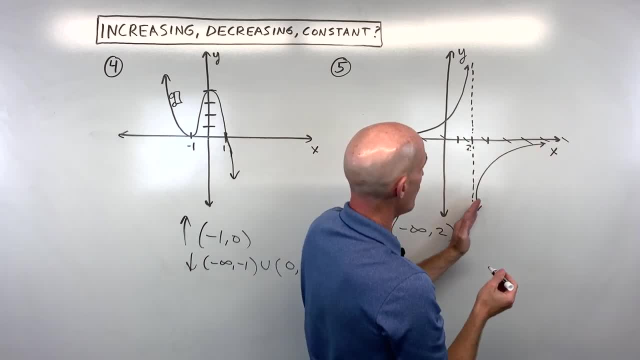 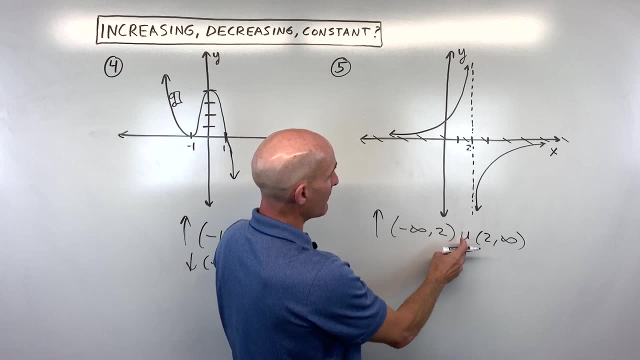 up, up to the right again. So that means, for what x values are the y values increasing? Well, again that's going to be from two, Two to pause and Finney. So we have a little gap here because of the vertical asymptote.